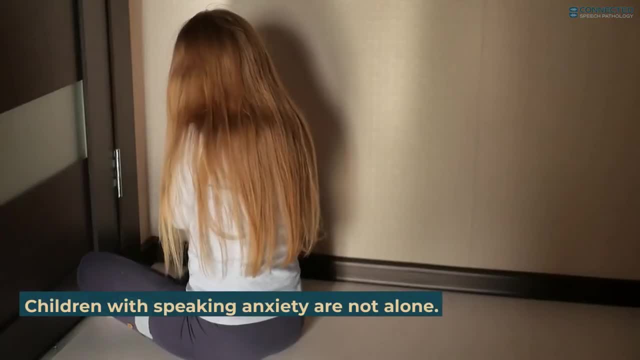 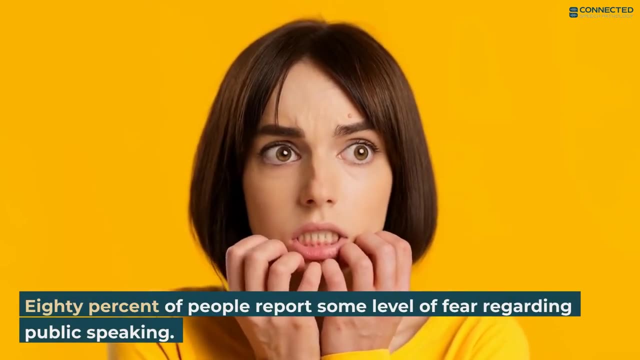 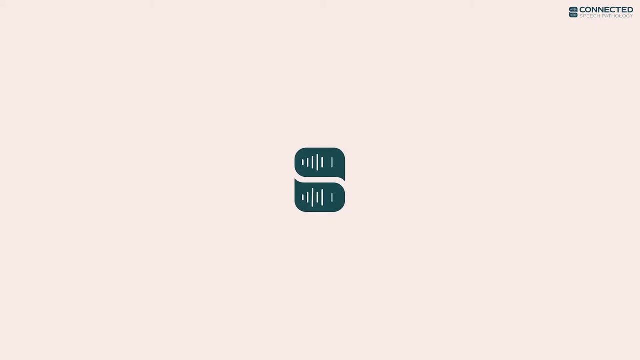 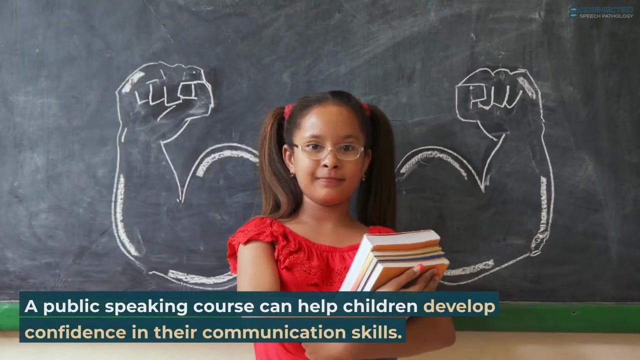 of anxiety and nerves. Children with speaking anxiety are not alone. 80% of people report some level of fear regarding public speaking. Public speaking classes for kids. What are public speaking classes for kids? A public speaking course can help children develop confidence in their communication skills. 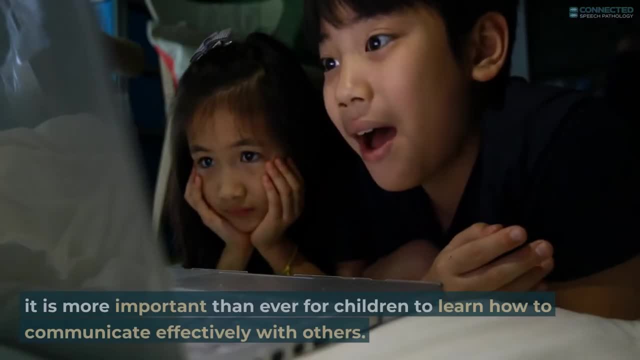 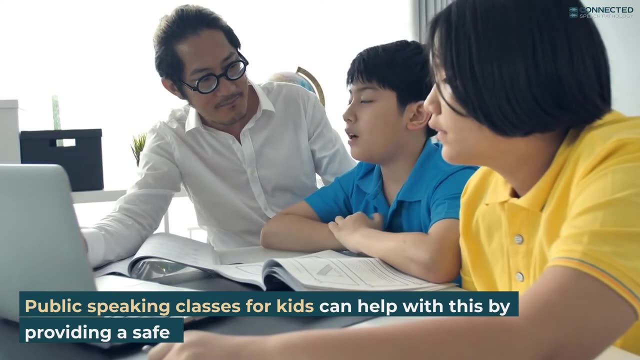 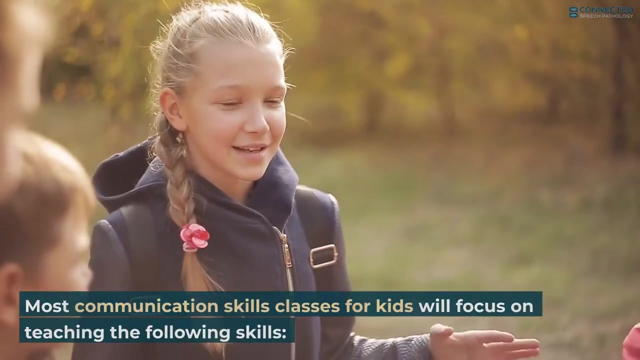 In a society that increasingly relies on technology, it is more important than ever for children to learn how to communicate effectively with others. Public speaking classes for kids can help with this by providing a safe and supportive environment for students to practice their communication skills. Most communication skills classes for kids will focus on teaching the following skills: 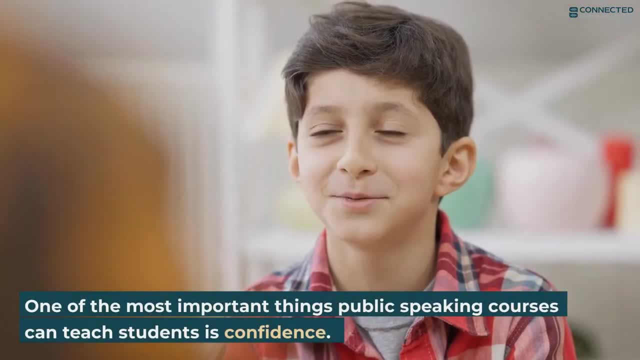 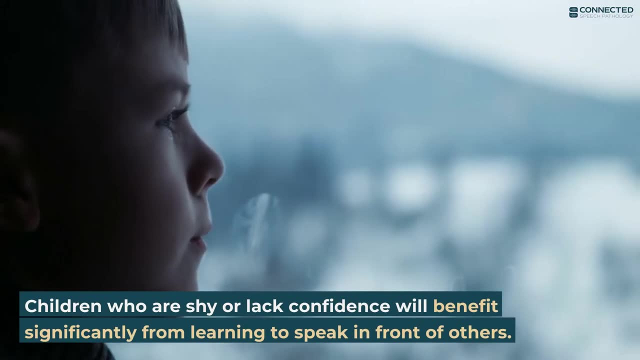 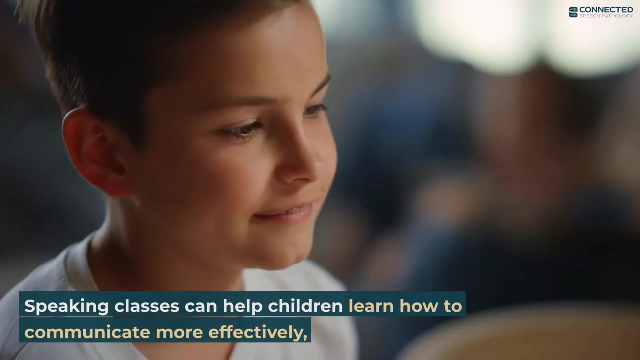 Confidence. One of the most important things public speaking courses can teach students is confidence. Children who are shy or lack confidence will benefit significantly from learning to speak in front of others. Communication skills- Speaking classes can help children learn how to communicate more effectively, including articulating their thoughts and feelings. 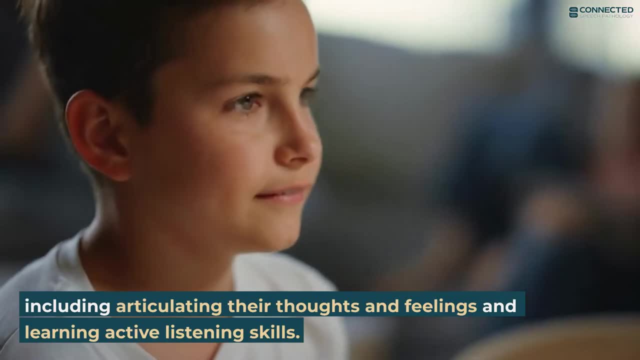 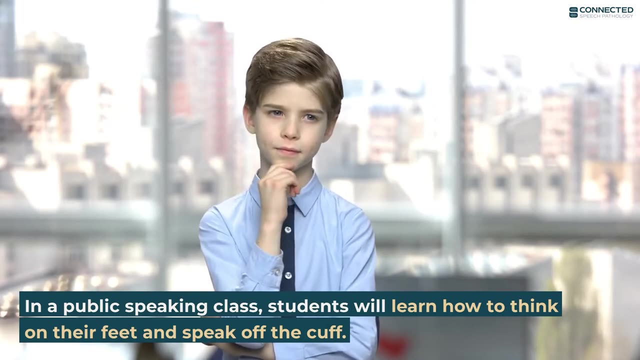 Learning to understand each other's feelings and learning active listening skills. Thinking on their feet. In a public speaking class, students will learn how to think on their feet and speak off the cuff. This valuable skill will come in handy in many situations, such as job interviews and networking events. 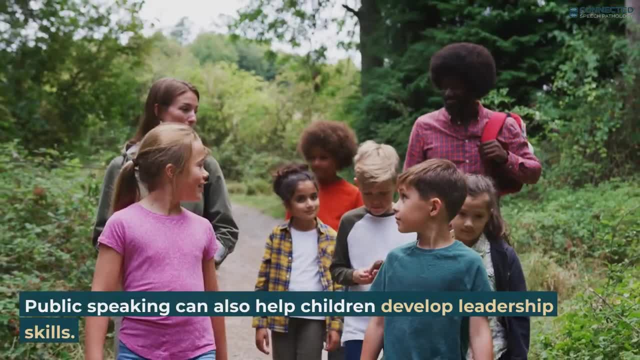 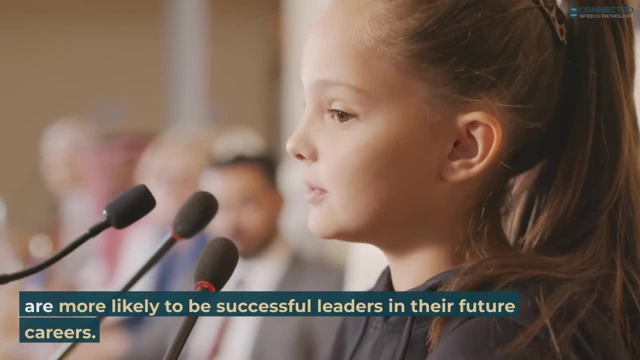 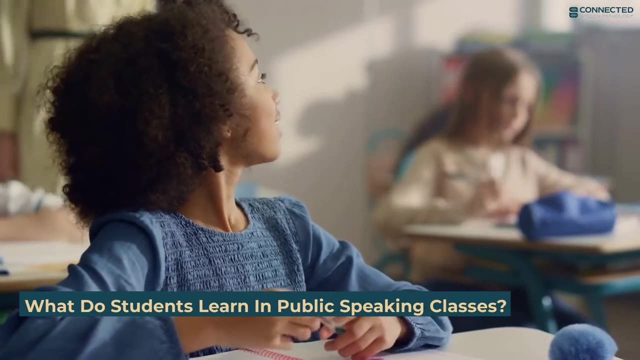 Leadership skills. Public speaking can also help children develop leadership skills. Children who can stand up in front of a group and give a speech are more likely to be successful leaders in their future careers. What do students learn in public speaking classes? In a public speaking course, students will learn to command attention. 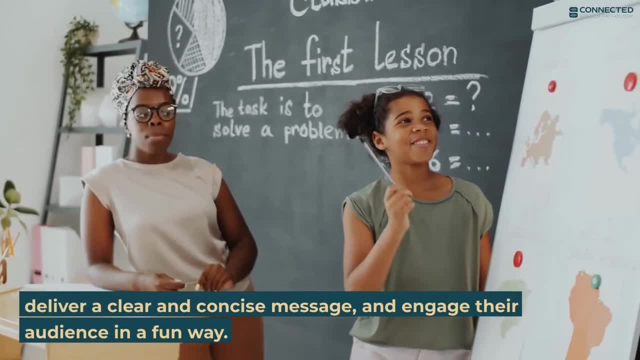 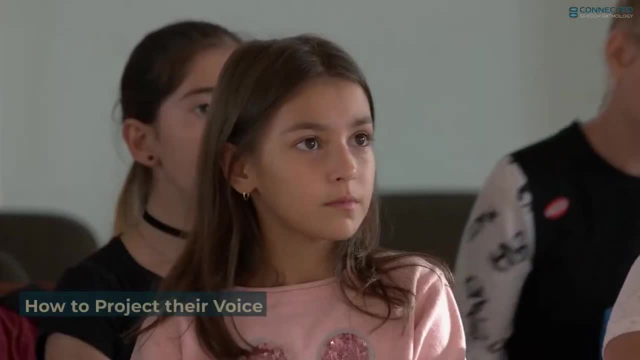 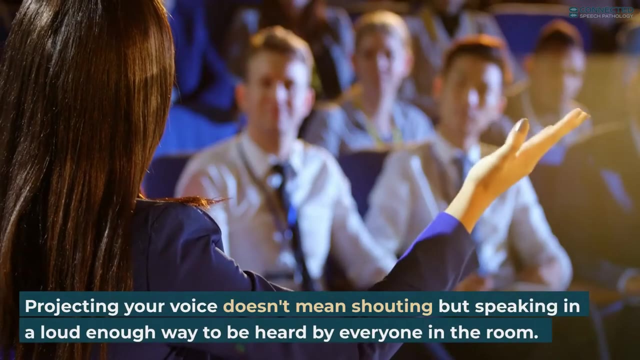 deliver a clear and concise message and engage their audience in a fun way. Here are some skills your child might learn in a public speaking class: How to project their voice. Projecting the voice is a challenge for many people. Projecting your voice doesn't mean. 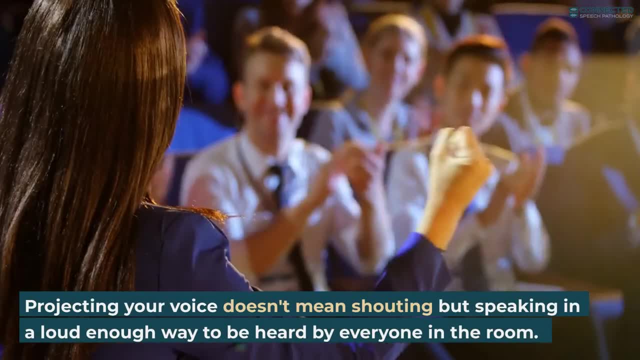 shouting, but speaking in a loud enough voice. Projecting your voice is a challenge for many people. Speaking in a loud enough voice is a challenge for many people. Projecting your voice doesn't mean a loud enough way to be heard by everyone in the room. 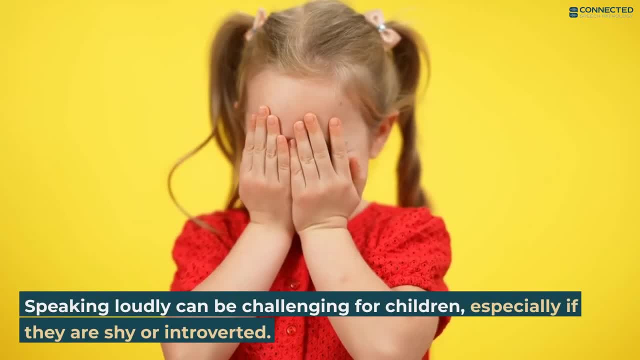 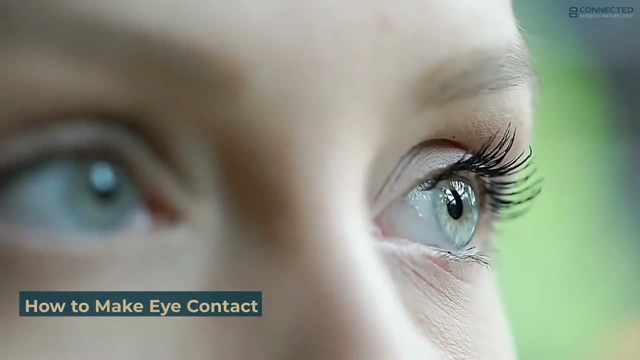 Speaking loudly can be challenging for children, especially if they are shy or introverted. However, with practice, it is a skill that can be mastered. How to make eye contact. Another essential skill that kids learn in public speaking classes is how to make eye contact. 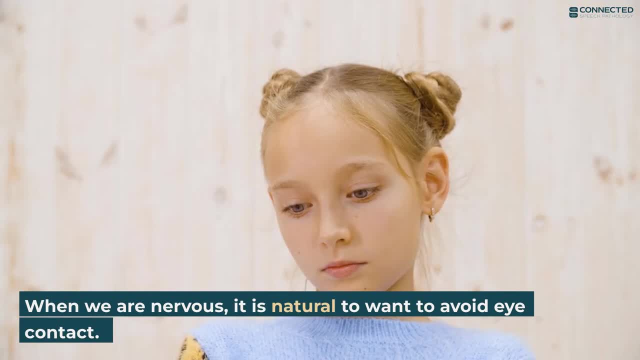 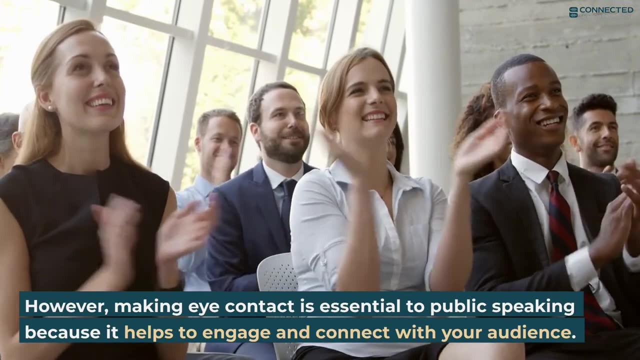 When we are nervous, it is natural to want to avoid eye contact. However, making eye contact is essential to public speaking because it helps to engage and connect with your audience. Children who can make eye contact appear more confident and are more likely to hold their audience's attention. 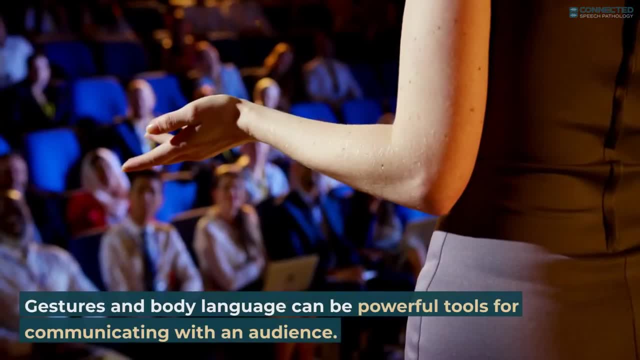 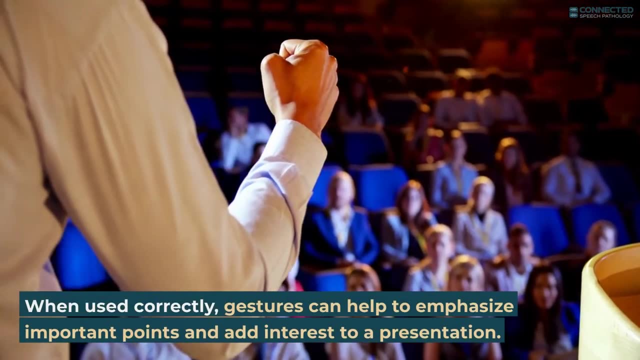 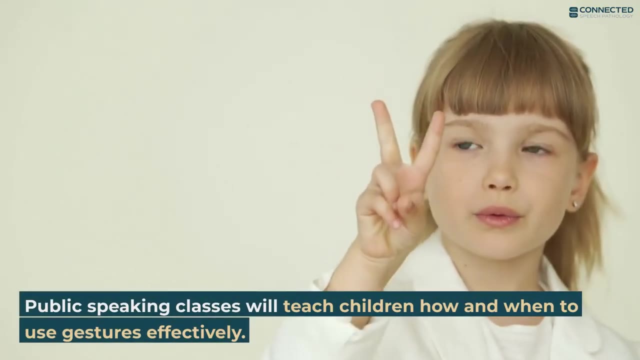 How to use gestures. Gestures and body language can be powerful tools for communicating with an audience. When used correctly, gestures can help to emphasize important points and add interest to a presentation. Public speaking classes will teach children how and when to use gestures effectively. 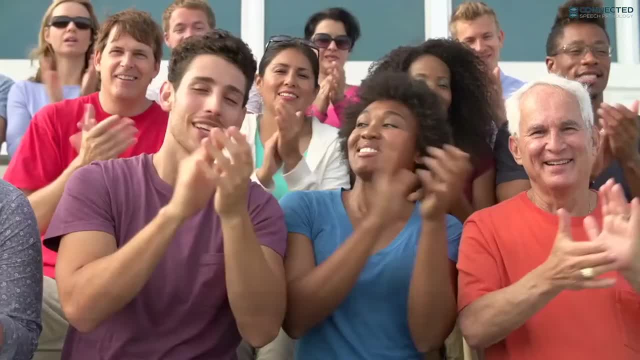 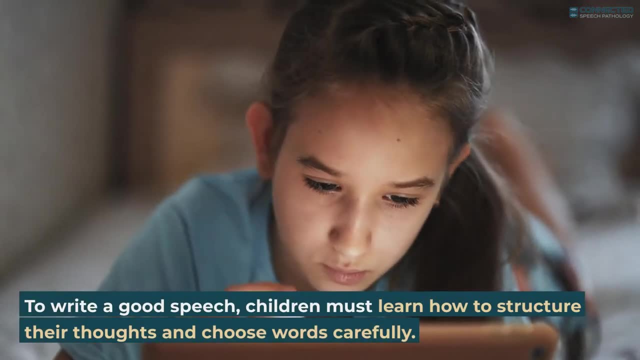 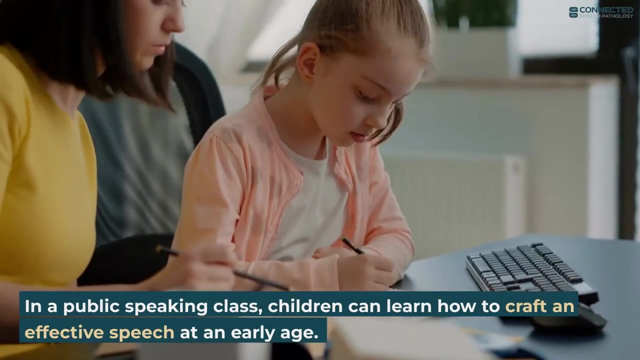 How to write a speech. A well-written speech is a key to delivering a successful presentation. To write a good speech, children must learn how to structure their thoughts and choose words carefully. In a public speaking class, children can learn how to craft an effective speech at an early age. 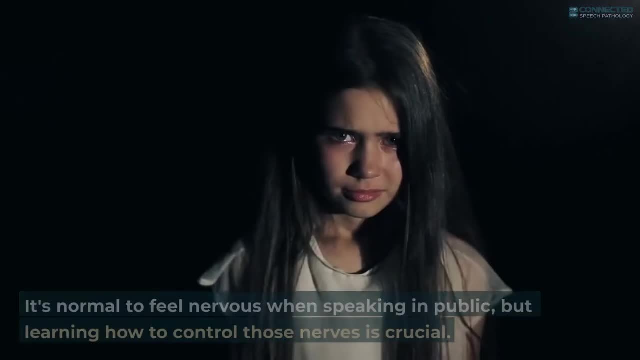 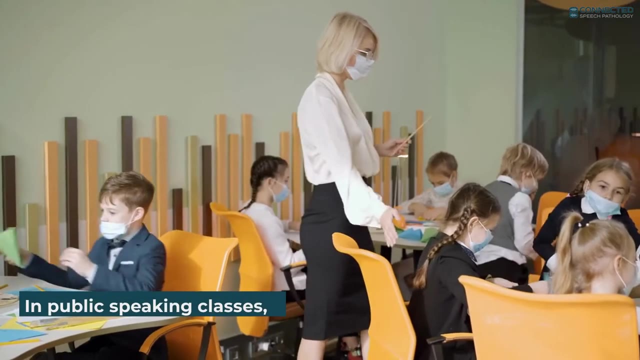 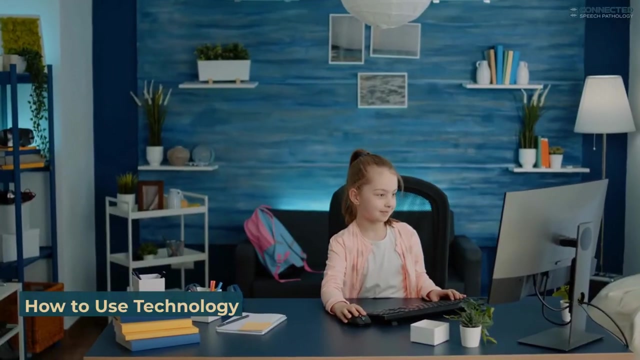 How to handle nerves. It's normal to feel nervous when speaking in public, but learning how to control those nerves is crucial. In public speaking classes, children will learn how to use these techniques to speak confidently in front of an audience. How to use technology. 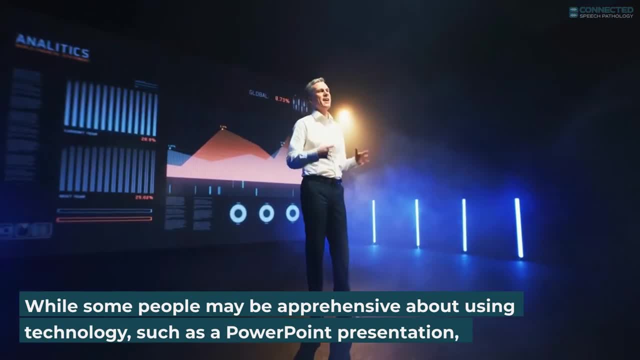 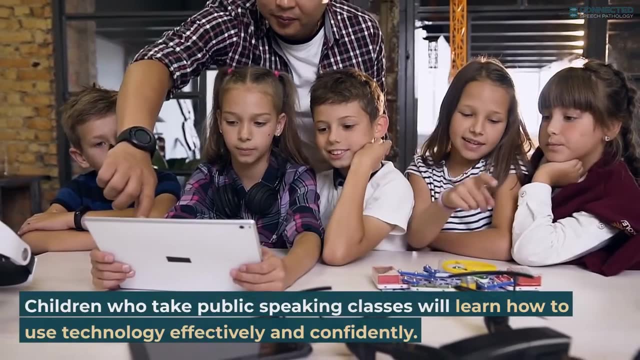 While some people may be apprehensive about using technology such as a PowerPoint presentation, it can be a great way to engage an audience and add visual interest to a speech. Children who take public speaking classes will learn how to use technology effectively and confidently. 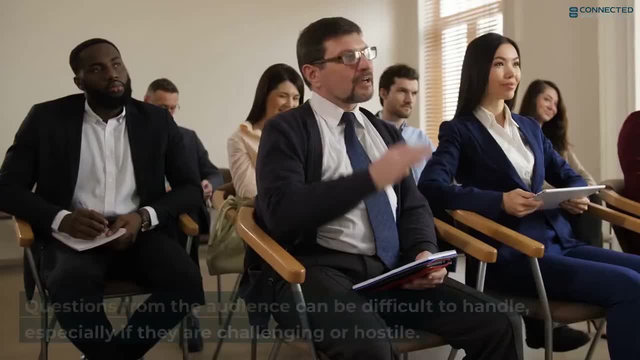 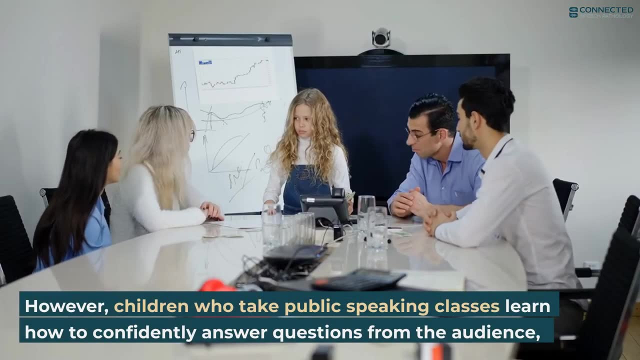 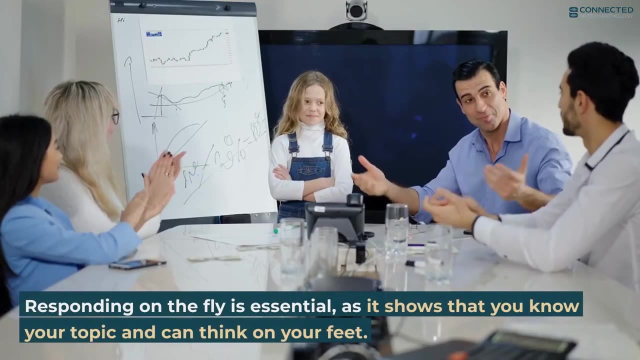 How to handle questions from the audience. Questions from the audience can be difficult to handle, especially if they are challenging or hostile. However, children who take public speaking classes learn how to confidently answer questions from the audience, no matter what they might be. Responding on the fly is essential, as it shows that you know your topic and can think on your feet.